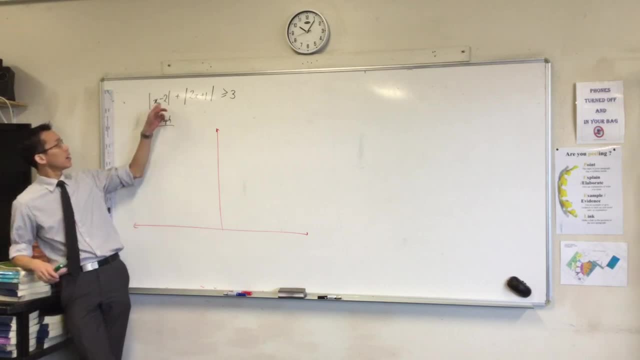 It's like it decepts the minus 2.. Yeah, And then it just keeps going. Yeah, it's just got a gradient of 1, right? So I have that visually in my mind. Is there a ruler here? Here we go. 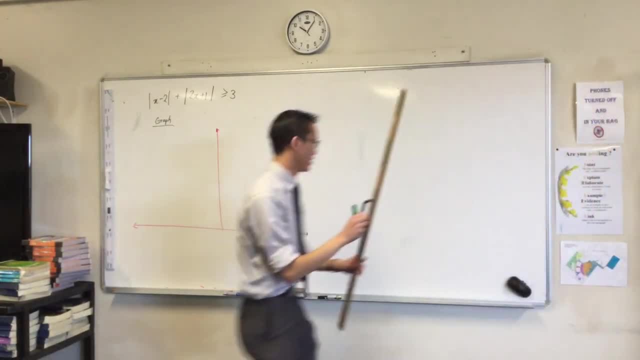 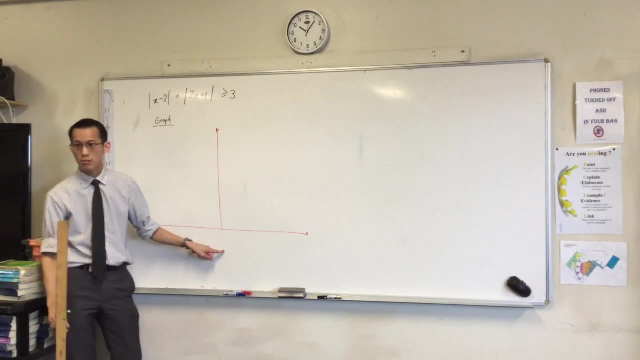 Oh, hidden up there. Yeah, I see, Okay. So it's where a teacher would hide it. You'll notice I haven't drawn the bottom of the axis. Do you know why? Because it's absolute values. It's absolute values. 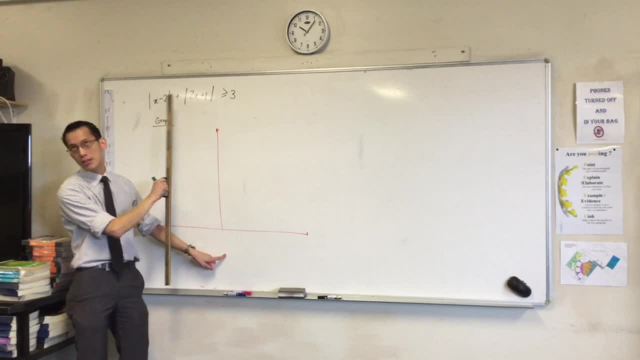 Not only is it absolute values, I'm adding absolute values. If you add two things that are positive, you'll get something else that's positive, So that's why I've ignored the bottom. However, it wouldn't do something like this, wouldn't it? 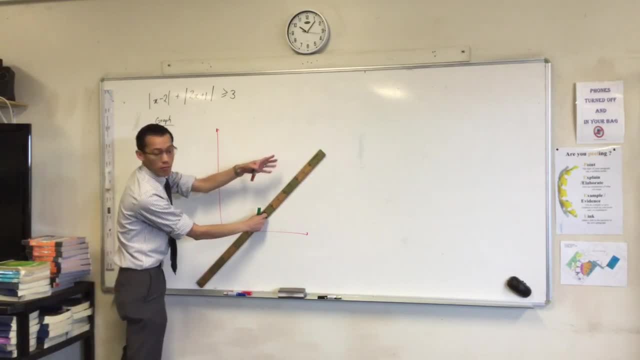 No, Okay, If that was like negative 2, and then off you go and your grade will be at 1, okay, So I'm going to be a bit cheap and I'm going to draw part of it right now. 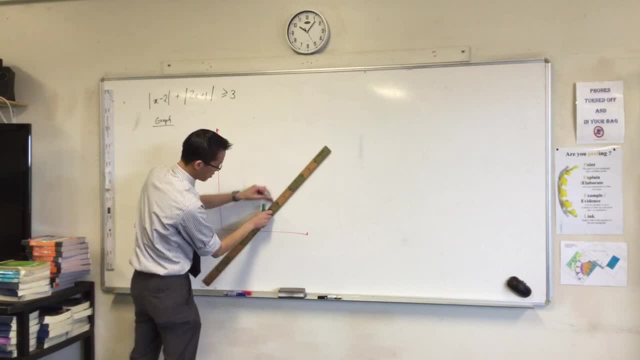 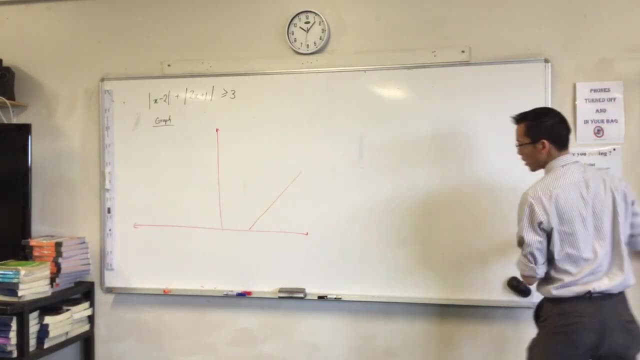 Like this, Move it over a little bit. actually, That is the only part that I've drawn, Because that's the positive part. the rest of it is irrelevant. Okay, What does happen to the rest of it? It bounces off. 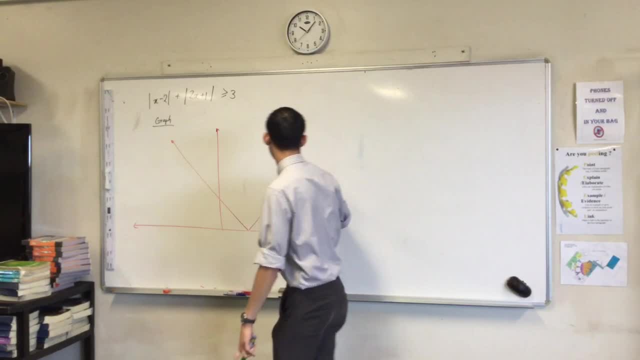 Yeah, very good, Something like that. Okay, So this and this is important. I've got two branches right, So I'm going to label the branches as they are. This part here is: y equals x minus 2.. What's the other part? 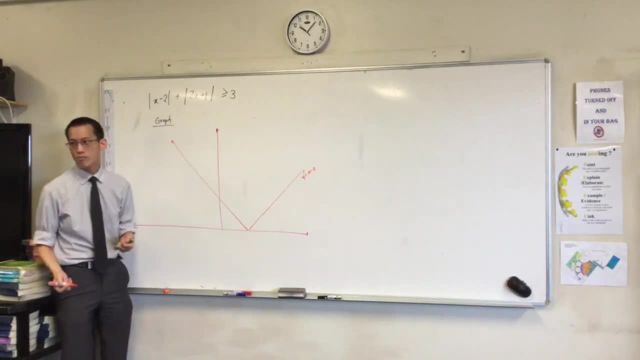 y equals x minus x plus 2.. No negative: 2 minus x. Either way is fine. I'm just going to write 2 minus x because I'm lazy and that's positive. Okay, But it's valid to say negative: x plus 2.. 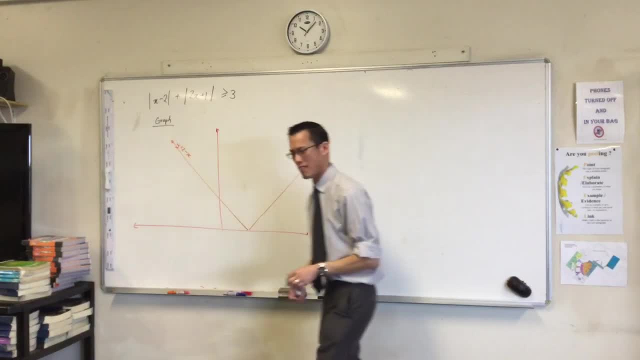 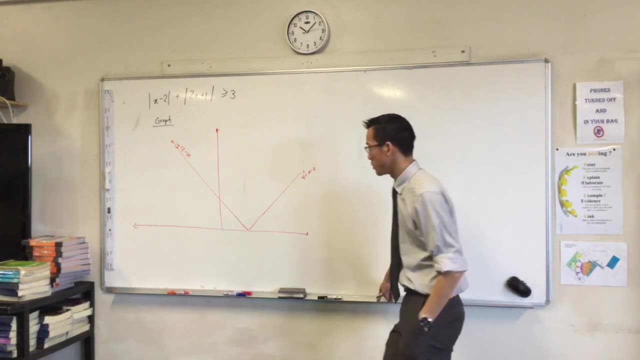 Cool, Now I've got the other part: Absolute value of 2x plus 1.. What can you tell me about it? The gradient of 2 crosses out 1.. Good, So, now that I have actual values on my graph, what is this value again, 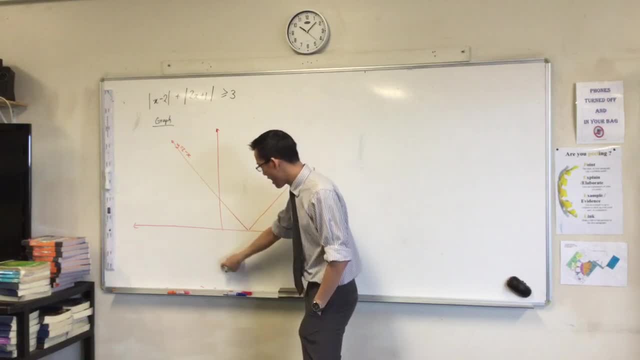 This one here. It was negative 2 and it reflected up to 2.. So if that's 2, then just for my own sake I'm going to put 1 in a reasonable spot. So there's 1.. So it crosses the axis there, and you told me it was steep. 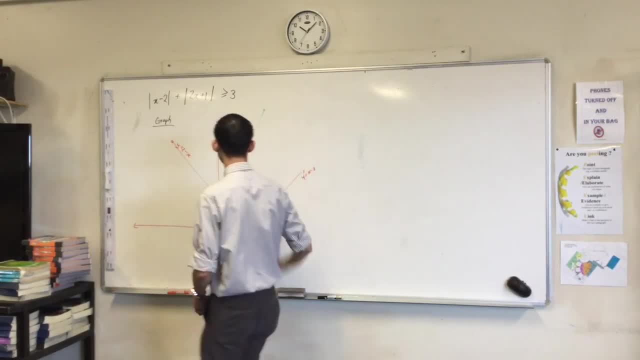 So it's going to do something like this. You okay with that? Then, of course, there's a reflected bit, So let's see how we go. That's too steep. I'm going to try that again. Like I said, I'll be a bit of a stick-over. 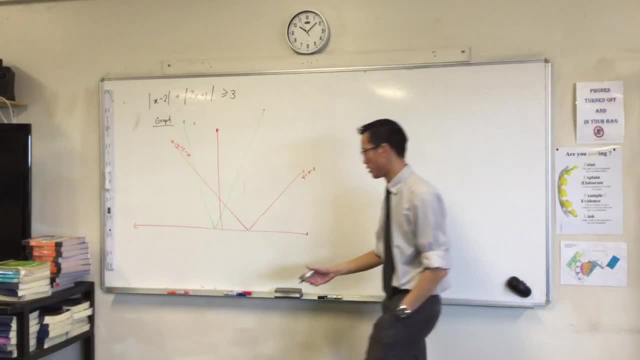 You only need it good enough to get a guy. Okay, Now again, this part has two branches, So you've got the 2x plus 1 branch. And then what's the other branch? 1 by 1 minus 2x. 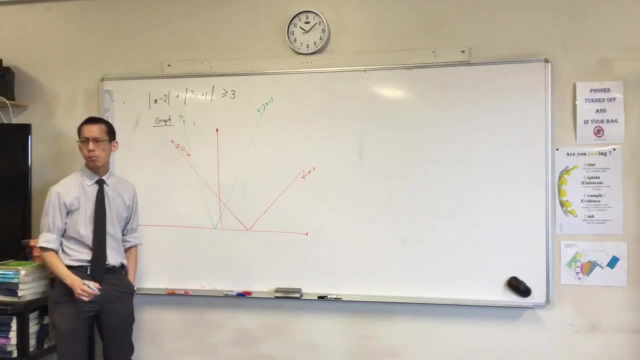 I'll be lazy: 1 minus 2x. Oh right, No, They're both negatives, aren't they? They're both negatives. The reason why this switched around is because 1 was negative and 1 was negative, Yeah. 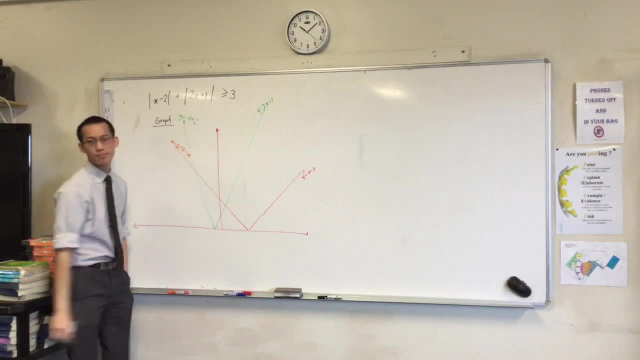 Big T spot. right, So this is, in fact, minus 2x minus 1.. You okay with that? Thanks, All right. So now we want to think about what this thing is going to look like Now. I already know a lot of places where the sum of these two graphs is going to go. 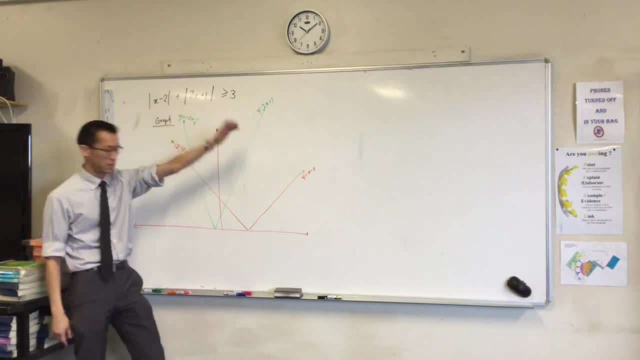 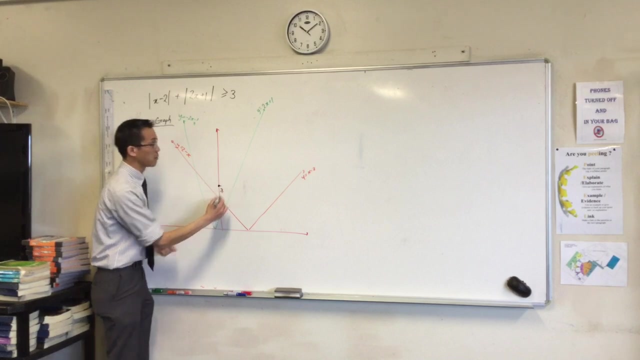 through. For instance, coincidentally, like I just wrote these numbers down, coincidentally- the y-intercept for both graphs together is going to be 1 plus 2, which is 3.. That point's really important to me because it's on the boundary. 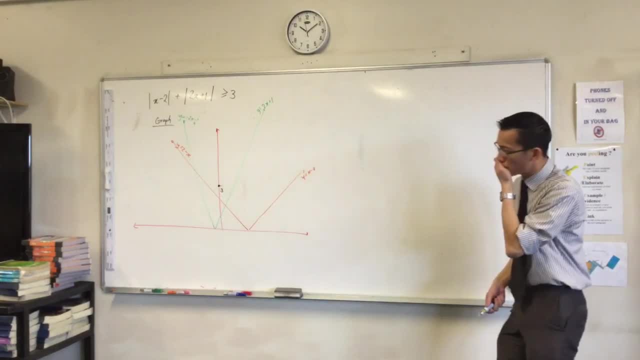 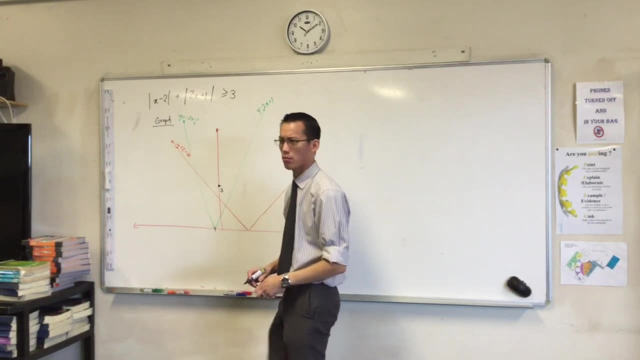 Okay, You can see there. all right, there's going to be to the left of this spot over here. By the way, what is that spot? Do you know what it is? To the left. To the left of the order. 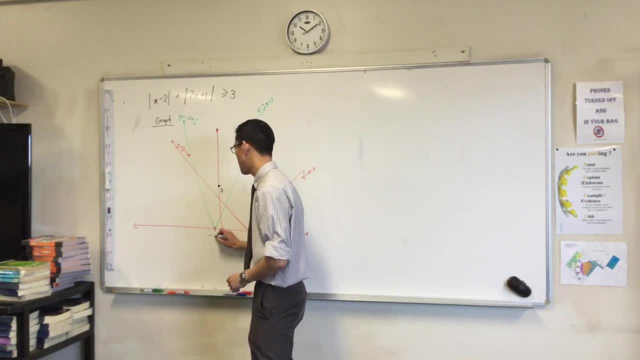 There's 0. 0. This is negative. It's going to be negative a half because, remember, it's got a gradient of 2.. So if you can imagine this little triangle in here with a rise over, run, that's half. 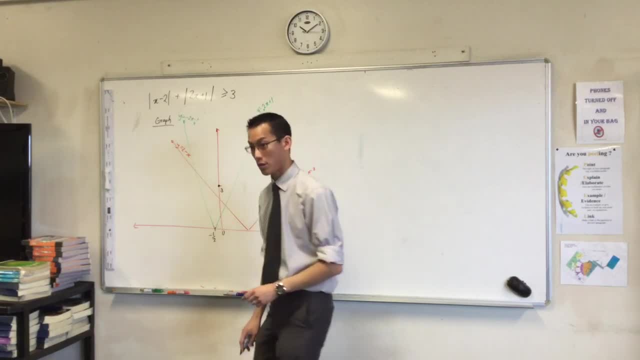 and that's 1.. So 1 divided by a half is 2.. There's your gradient. So to the left of this you're going to add these two guys together. All right, I'm going to go up on my graph to here roughly. 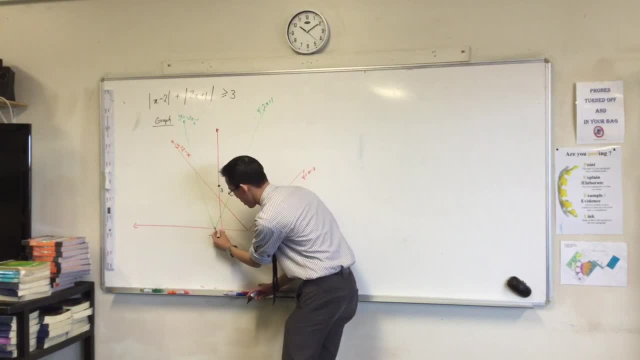 Now, how many of you are looking at this graph? Okay, So I'm going to go up on my graph to here roughly. Okay, Now, how many of you are looking at this graph? All right, All right, All right. 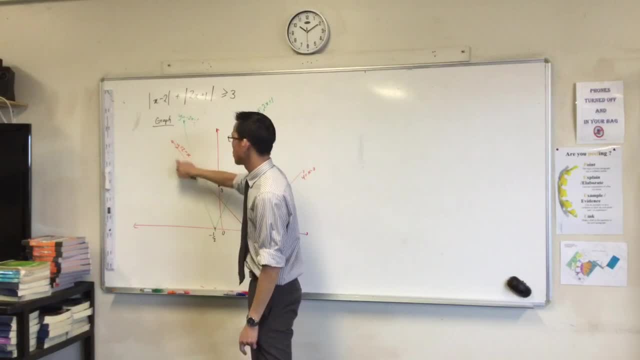 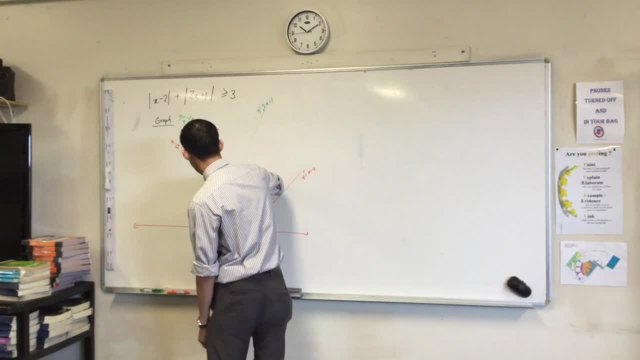 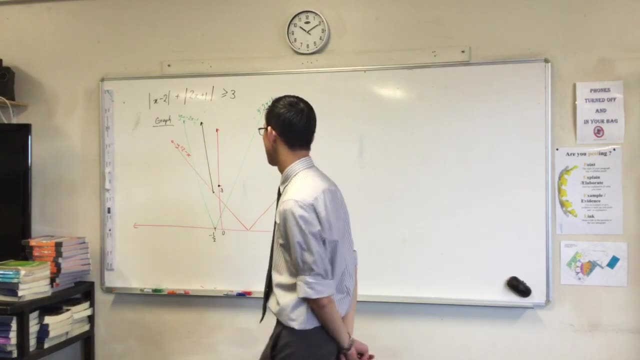 One, One, Yes, Yes, that's what I expected. You're going to have a line that's really really steep. Wait, So can you Right up there? So… Yep, Right up there. So the negative half the…. 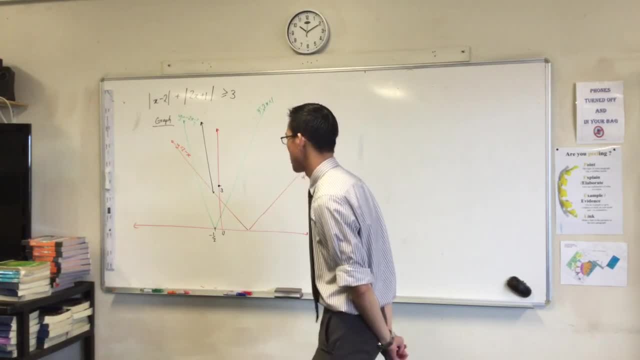 Yep. How did I get it? Where did they come from? It's just because of the… So I can think of it in terms of gradient. That's one way to think about it. Another way to think about it is…. It is the junction where the…. 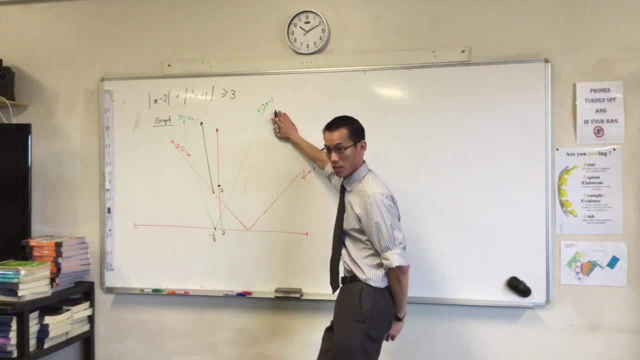 The gradient, This branch turns into this branch agree. And the junction is: is this thing positive or is it negative? right, It changes exactly when it's zero. So I can do this, which gives me this. So that's what gives me this. 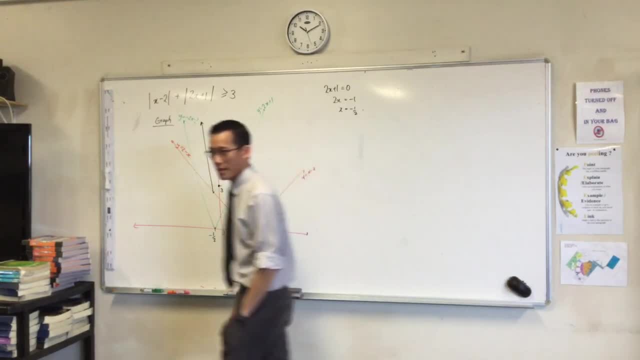 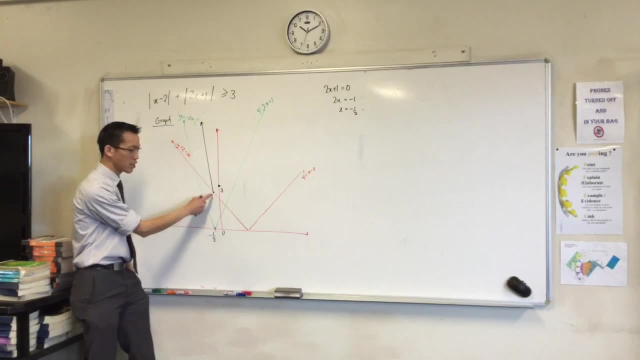 And how do you move it up? and then like the dot and then Yeah, yeah, yeah, OK, So at this point here the green graph is zero, And then I'm adding zero to something else. I don't know what the something else is. 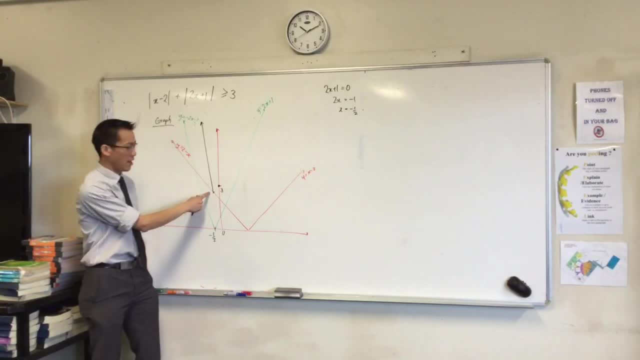 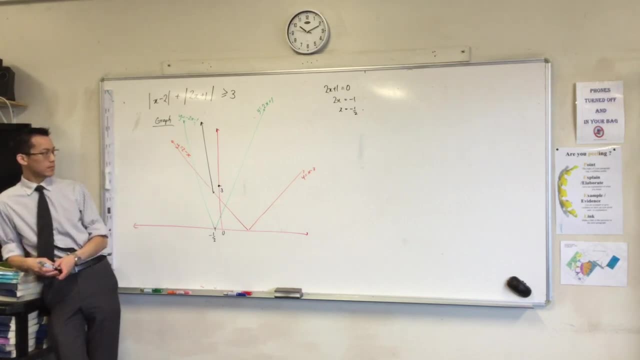 but zero plus something will be something right. Something just below three, between two and three, The absolute value of x. it could be off the x-axis, right Off the yes, absolutely. So then how would you do that? 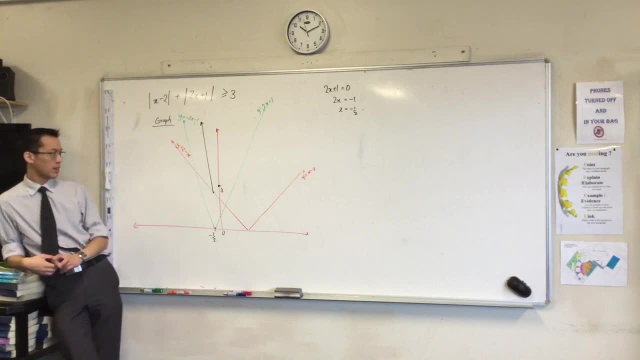 Do you want me to do that as a separate question? Yeah, I can do that, that's fine. For now, though, I can sort of address the skill you need for that question, Even with you. I'll give you this question. I'll show you what I mean. 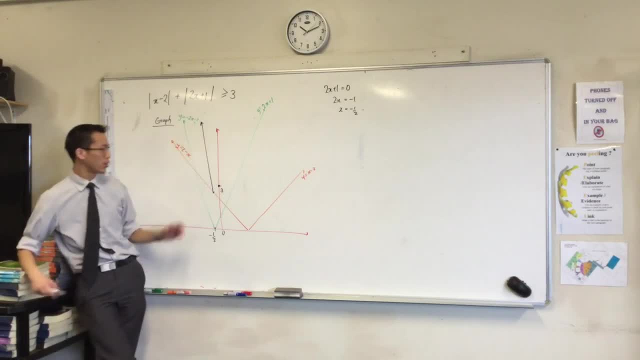 What have I got here? OK, this line is really really steep Because you've got this decreasing line. I'm reading left to right, This decreasing line and this decreasing line, So they're both decreasing. It's really really decreasing. 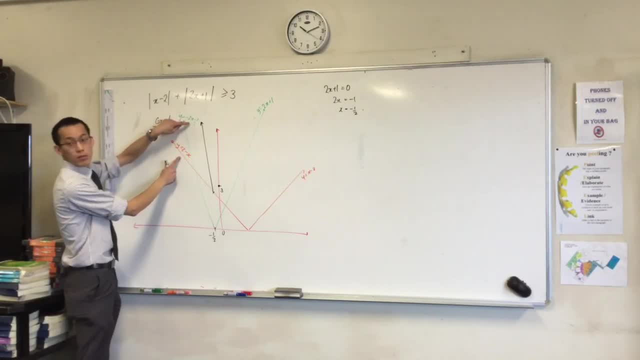 I can find out how much it's decreasing by looking at these two formulas and adding them together. the equations, right, It's going to be what's the coefficient of x? It'll be negative. three right, Negative two here and negative one here. 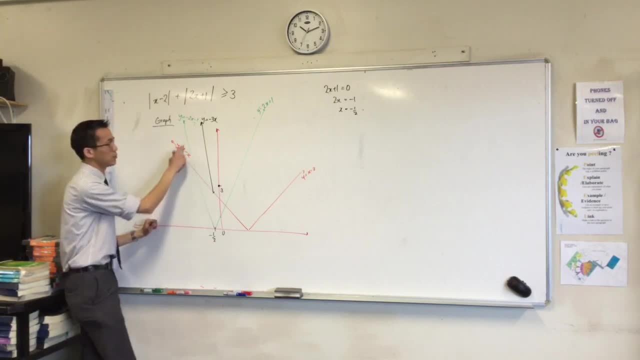 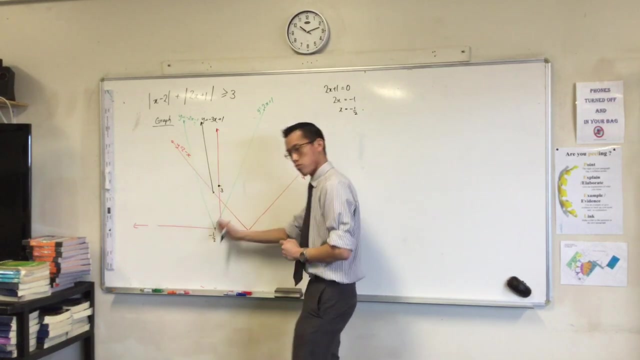 What about the constant Two? negative one, That's plus one, isn't it? So that's the branch, That's the equation of that mid-tall branch. All right, That was that. looking to the left of there, Then on the right, all the way up until here. 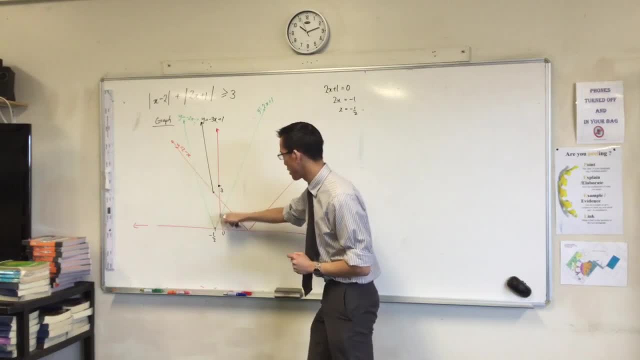 in this region. here this orange line is doing the same thing and this green line is doing the same thing, So I want to know what's happening in between. What's this value? Two, Very good. So between negative 1 1⁄2 and two. 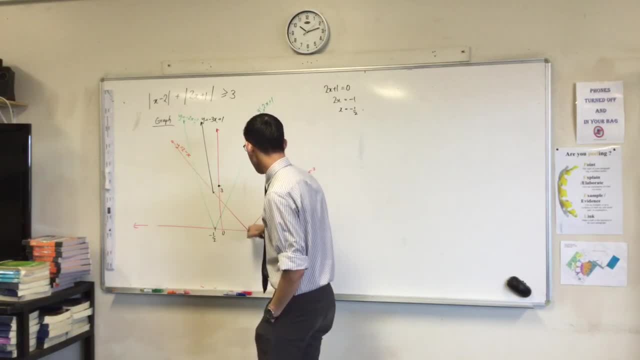 you've got this line that's going down. You've got zero plus this, Zero plus this, whatever this is. So zero plus this is just yeah, OK. And in between you've got a point here We already know the y-intercept. 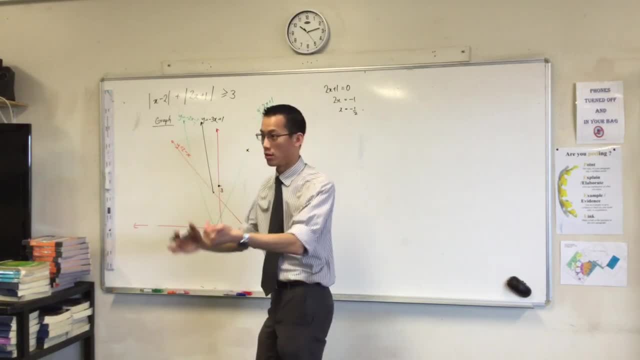 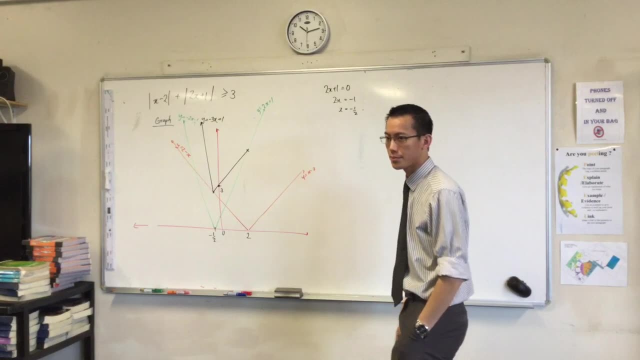 Another point: These are all straight lines. You add straight lines, you get more straight lines. So this is the thing that joins all of them, Basically anything in between. There you go, There you go, There you go. The value is always a straight line. 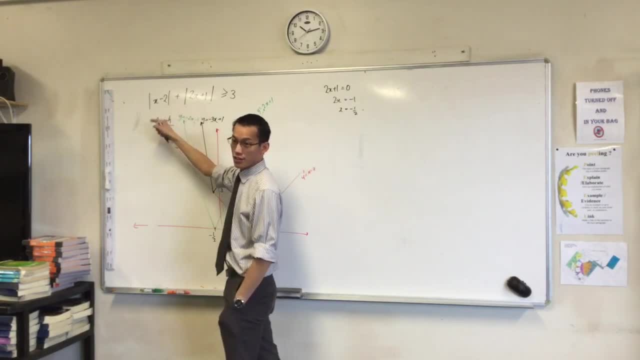 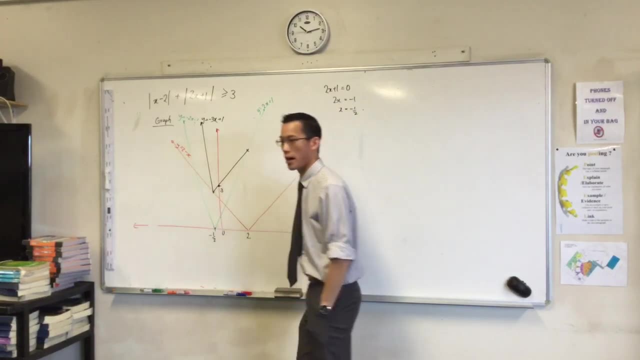 Yeah, that's right. The sum of linear functions is another linear function is the way we would say it. All right, Now again we can work out the equation of this middle part. How are we going to do it? Add the decreasing branch with the increasing branch. 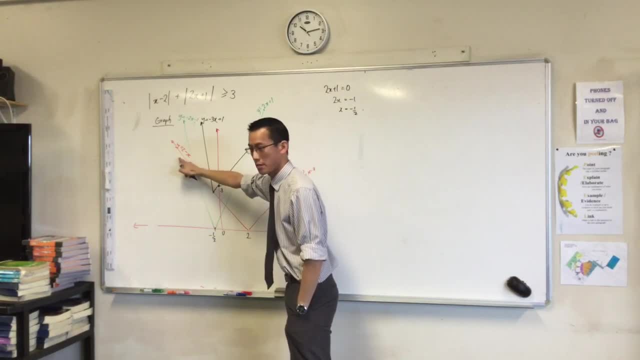 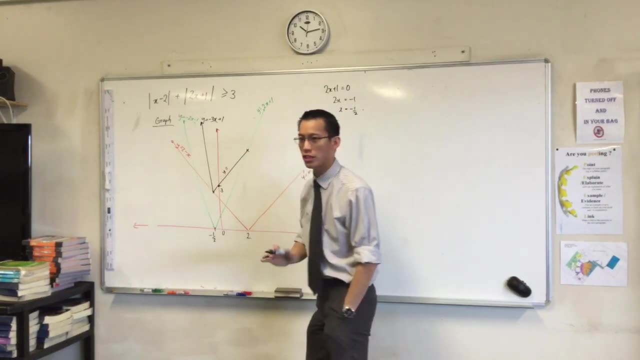 Very good. So this orange decreasing branch is 2 minus x, But this green increasing branch is 2x plus 1.. So y is going to be equal to just collect the like terms, the like terms for x Plus 3.. 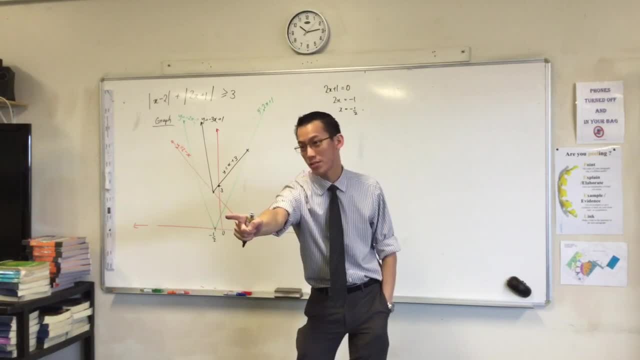 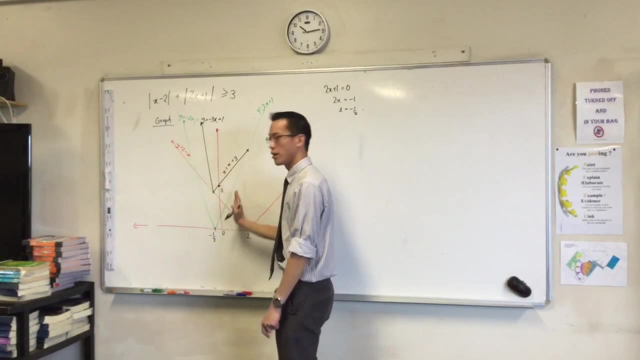 Yeah, Perfect, And you can know it's x plus 3, because, look, it goes through 3.. Yeah, We already worked that out before. And the gradient of negative 1, the gradient of 2, that leaves you with a gradient of 1 when you add them. 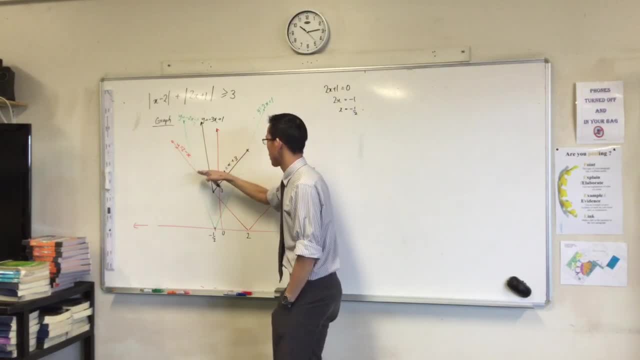 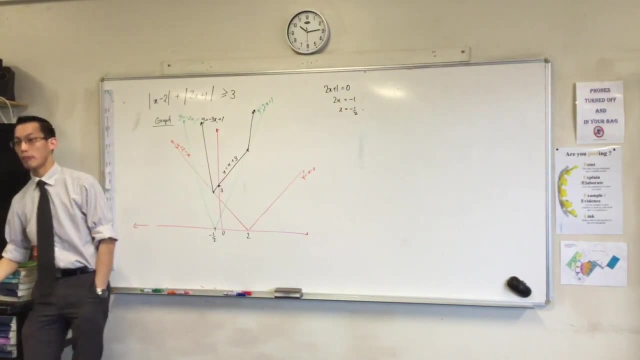 OK, Now watch this. See how I've been carefully constructing each bit, working on what the equation is. I'm going to draw this bit and then I don't give a rip what the equation is. This is one of the great things about not doing it in three cases. 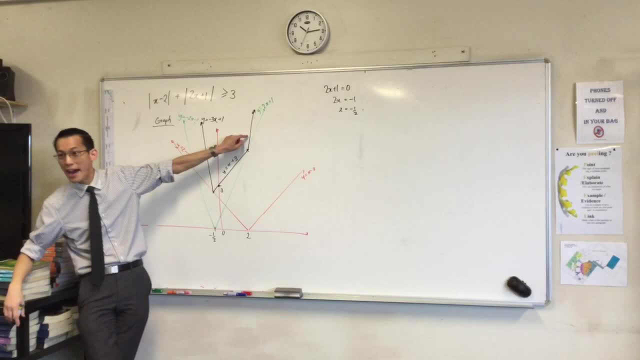 Because once you draw the graph, you're going to get a point. You're going to get a point, But if you look at the picture, you know this part doesn't matter Why? Because it's already above the 3.. I'm already above 3.. 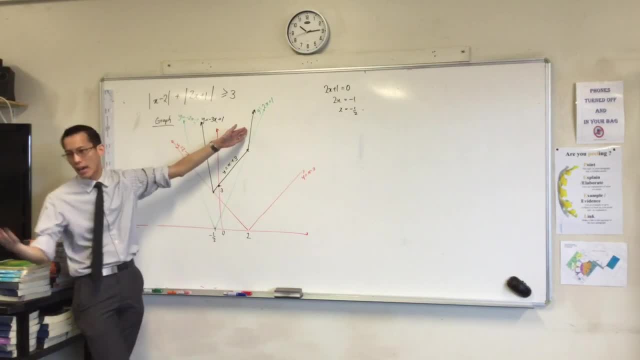 Right, I already went above 3 here, So I don't care. I mean, I can't work out this equation, But I never need to touch it, Never, ever. OK, All the interesting stuff is happening in here, So that's enough of a graph to do this. 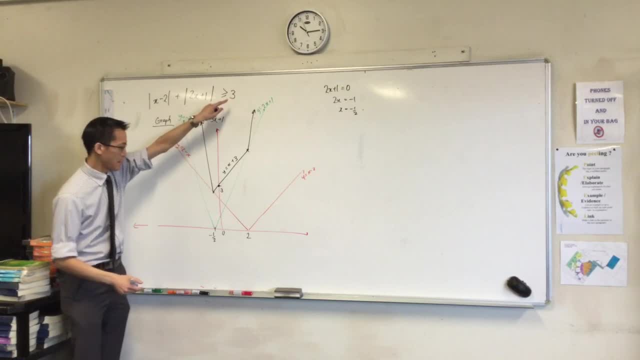 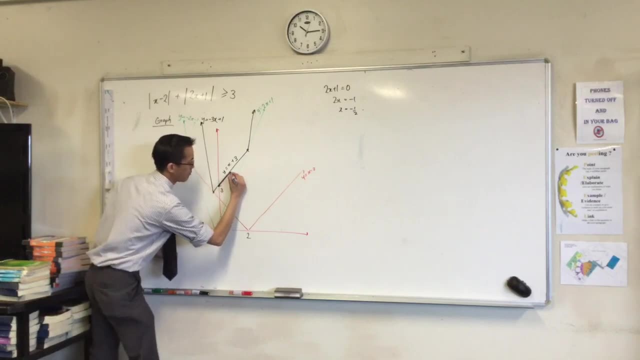 I need to work out the parts that are above 3. There's only actually a small component that's below 3. Right, This part here. that's the dud Right. So from here upwards is good, And then from here upwards is also good. 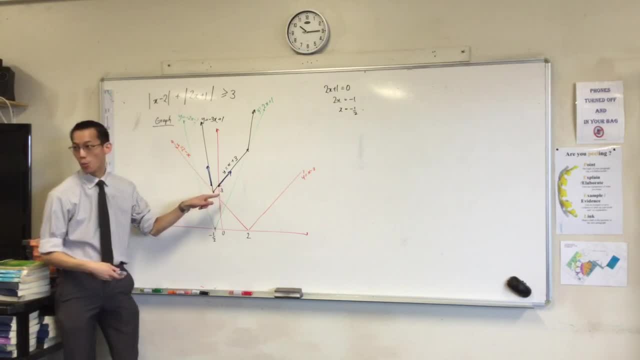 Right Now. conveniently, this has landed on the y-intercept Right, So that's where x equals 0. So this is just going to be: x is greater than or equal to 0. That will give me all those values. 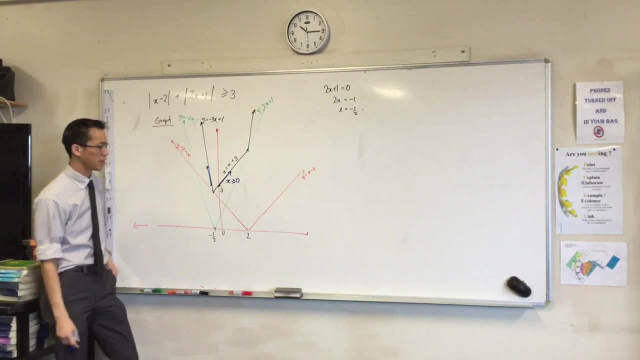 OK, This one is a bit trickier. How do I work that out? You have to substitute in. I'm going to have to substitute in. I know what the y-value is along here. It's 3.. Right, And I know what the equation of this line is. 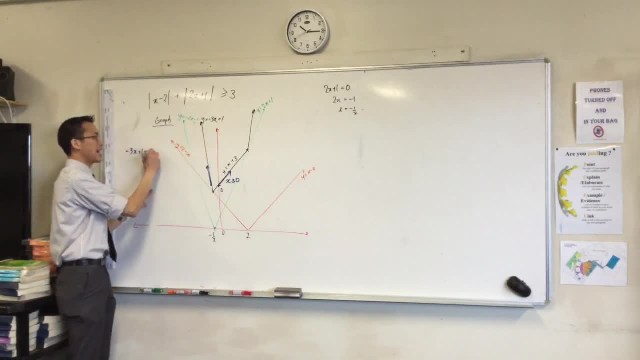 It's minus 3x plus 1.. So I'm going to say minus 3x plus 1.. Well, when is that equal to 3?? And the answer is: 2x equals negative 2 thirds. Does that look like negative 2 thirds? 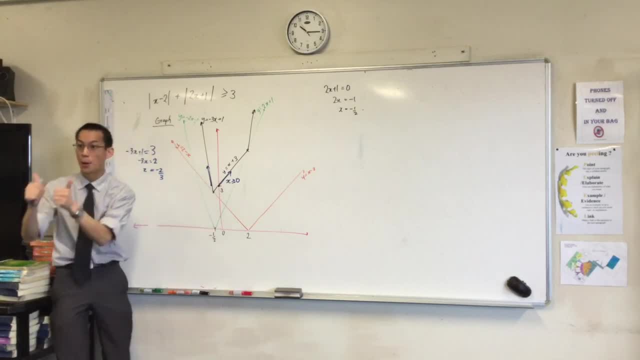 Yeah, Yeah, Look, remember that one That's negative 1 half. It's just to the left, Perfect. So this is: x is less than or equal to negative 2 over 3.. I've done all the legwork. 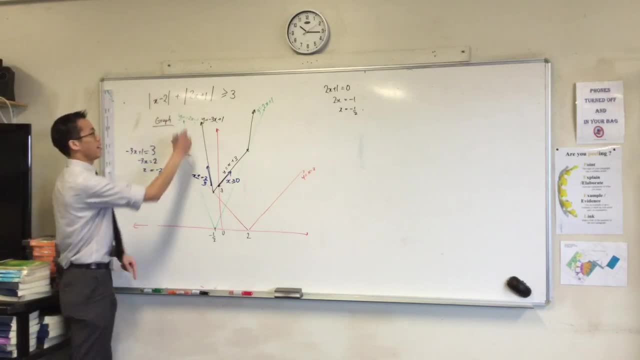 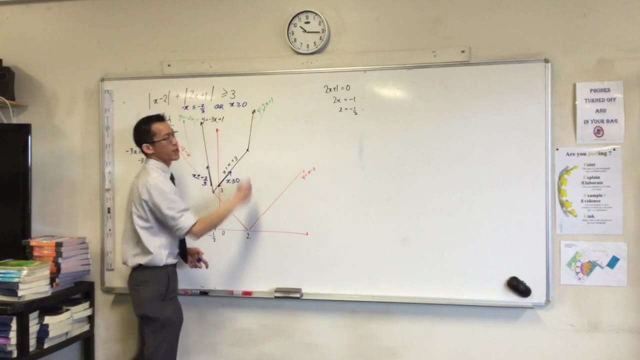 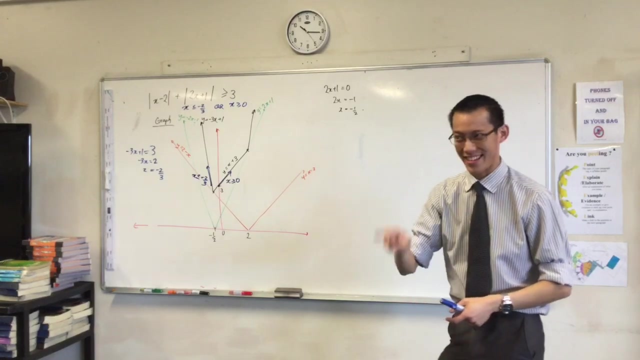 So now I can say: this is true when x is less than negative, 2 over 3, or x is greater than or equal to 0. Why is it or and not? and Because you can't simultaneously be greater than 0 and less than. 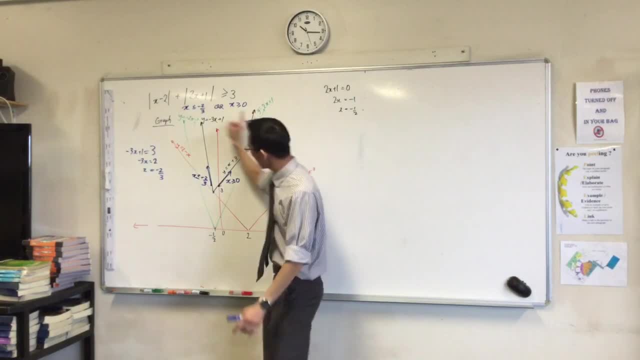 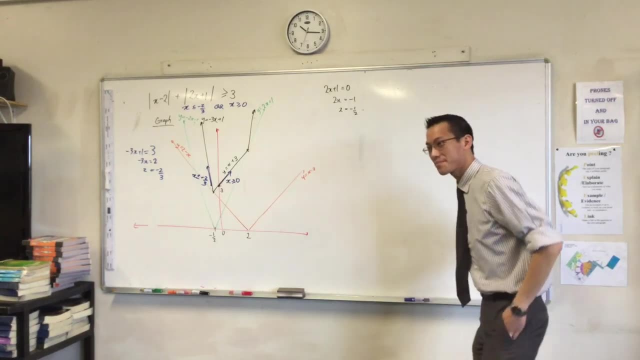 Yeah, There's no number. There isn't any number that can do both of these at the same time. You can be one or you can be the other, which is great, But not both. I didn't write anything in the first exam and I lost the mark. 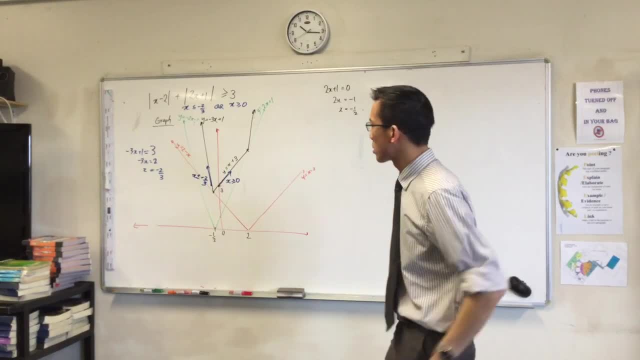 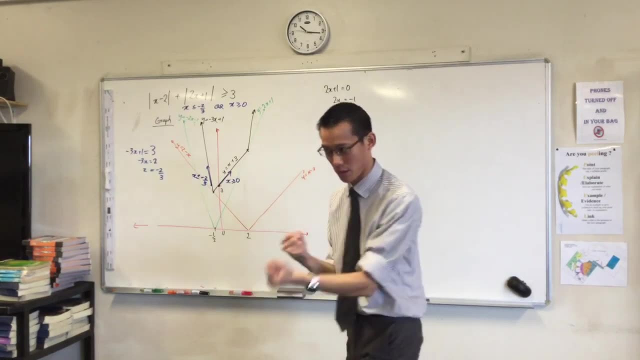 because I didn't have and or all and I meant to join them. Yeah, Well, sometimes, yeah. You see, this is one of the superpowers of mathematics, which is a two-edged sword. In mathematics, there's no wasted words. 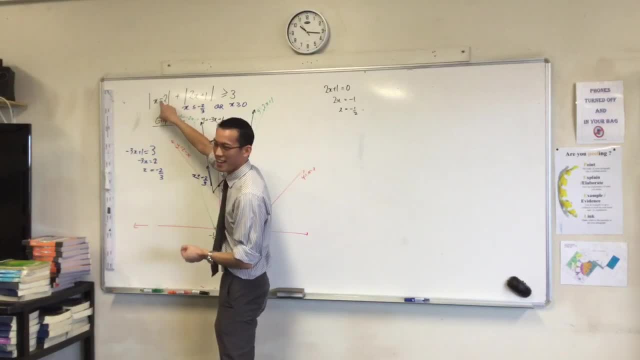 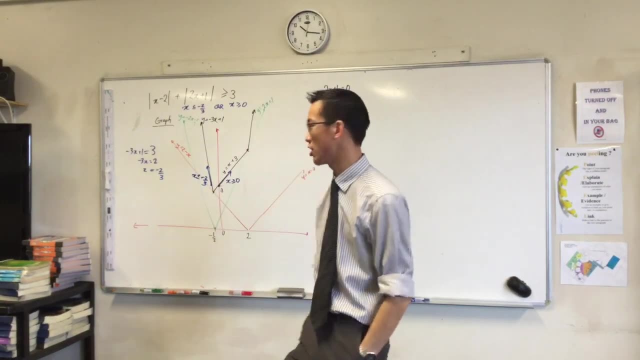 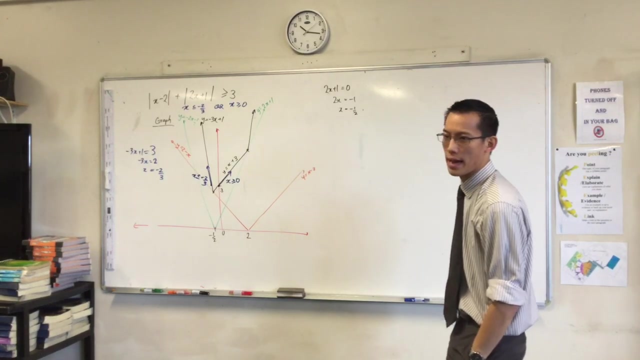 There's no wasted symbols. A single character changes everything, So therefore a word really matters. So economy makes things faster. It makes things faster and more efficient and more dangerous when you leave out little things. So if you were to do this by cases, OK, it's still doable.